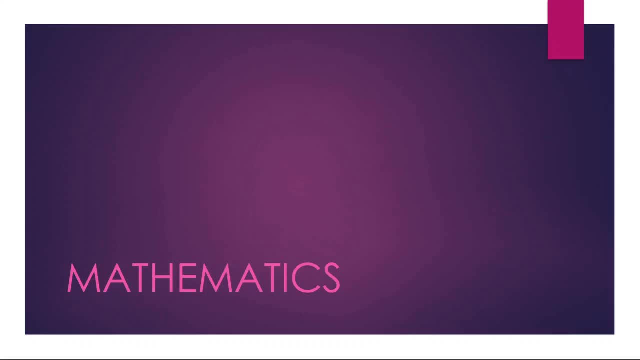 Hello, let me introduce myself. I'm Christina Hunt. I'm one of the math instructors here at Stark State. Today we're going to be looking at the mathematics portion of the Accuplacer. Now for the Accuplacer. the math part section consists of two parts. 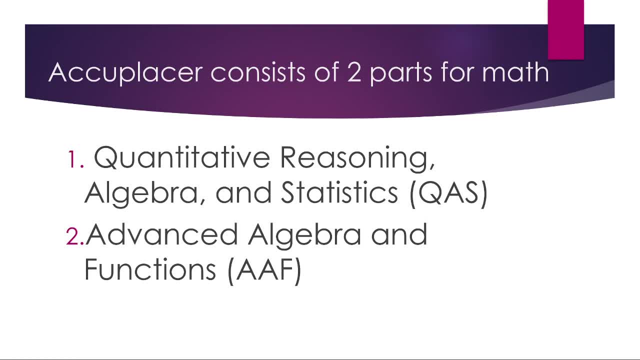 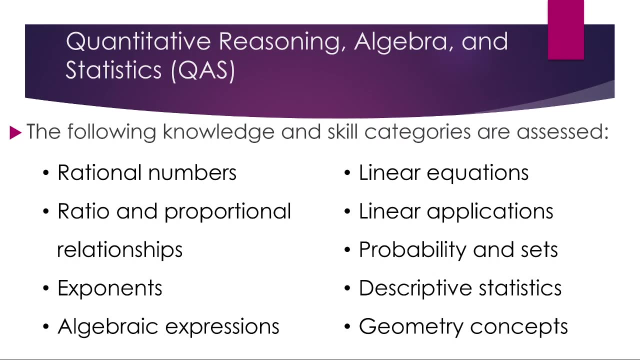 The first is one that's called Quantitative Reasoning, Algebra and Statistics. The second one is called Advanced Algebra and Functions. All right, we're going to first off look at the Quantitative Reasoning, Algebra and Statistics. This is more of the basic math portion. 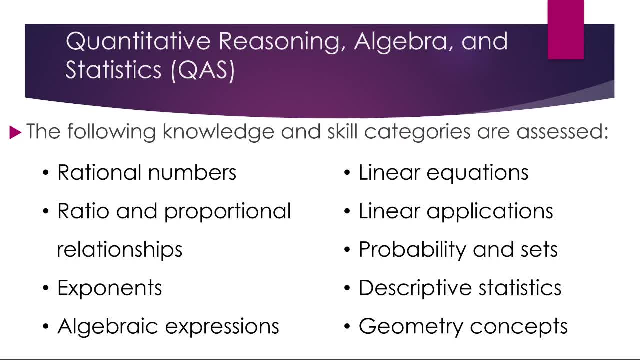 All right, you're going to be looking at things you possibly would have learned in algebra and geometry- topics like this. So you're looking at your rational numbers, your ratio and proportions, exponents, basic algebraic expressions, some linear equations got in there, some applications. 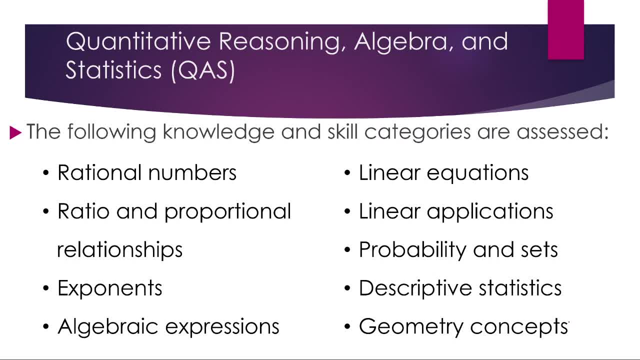 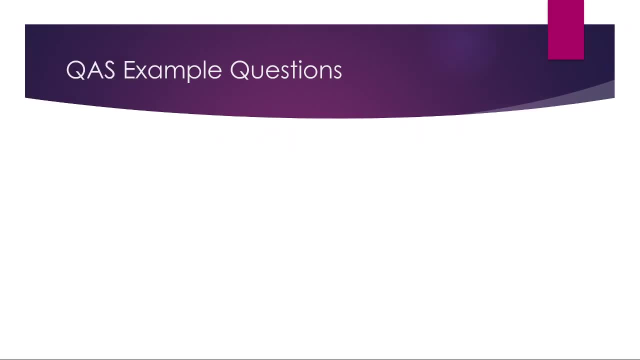 Some basic pieces from probability or descriptive statistics and some general geometry concepts, So things that you would have learned at the beginning of your high school career. We're going to do several examples here just so you get a feel for what basic kind of things are in here. 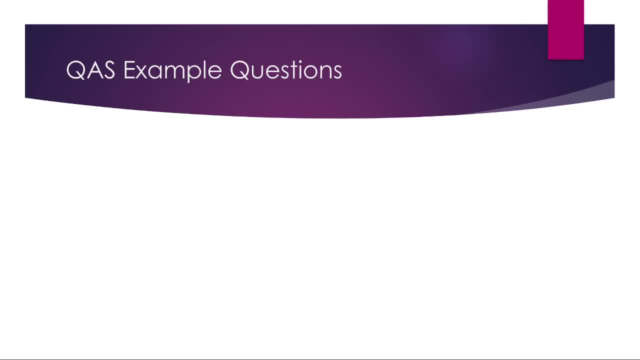 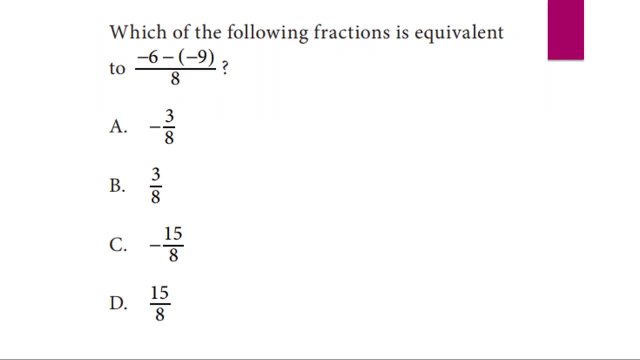 The examples did come from Accuplacer itself, So these are some of their example problems. This first one starts off as just a basic problem. Okay, you're just going to have to simplify a fraction, All right, so this is testing. really, if you look at it, 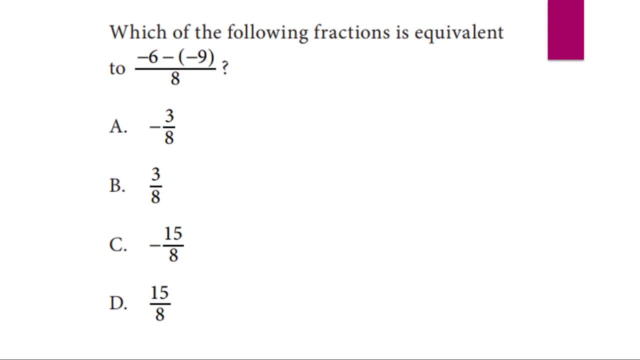 The big thing this is testing is the concept of my do I know how to deal with negative values? All right, so you should note right off the bat here. For this example- So this one- we have two negatives sitting side by side. 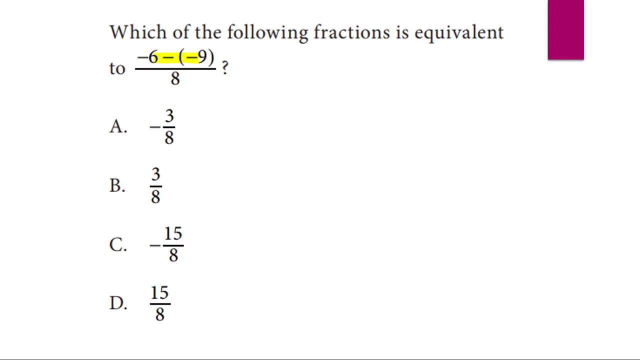 Any time I have two negatives, we know that two negatives make a positive. So that means my problem changes to a negative six plus a nine over eight. Then I have to remember my rules for dealing with unlike signs. So that means that if I have a negative six plus a nine I'm going to subtract the two values. 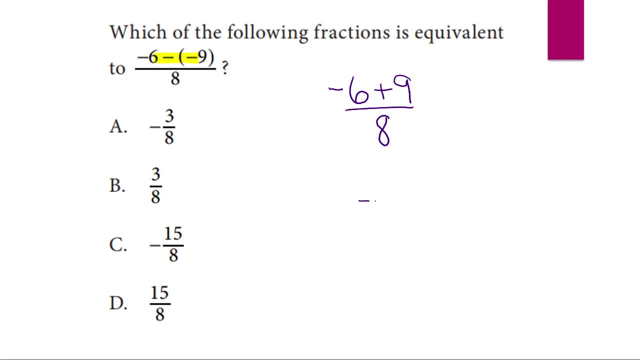 keep the sign of the larger, So a negative six plus a nine. So nine minus six gives me three. The sign of the larger would be the positive value, And then the eight still goes on the bottom. So my answer to this one would be B. 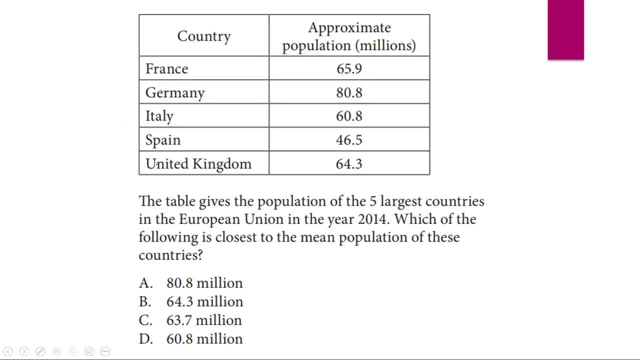 We started off easy. This next one is something you should have learned in numerous math classes. It's also found at the beginning of every statistics course in the world, And that is asking you to find the population mean of a group of countries. Now, any time we're trying to find a population mean, 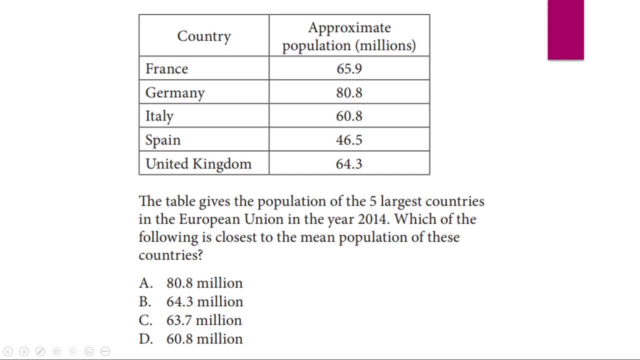 that means that the first thing we're going to do is we have to find the sum- And that symbol means sum- of all of our X's. Then we're going to divide by The number of items that we have. So the first thing I have to do is find the sum. 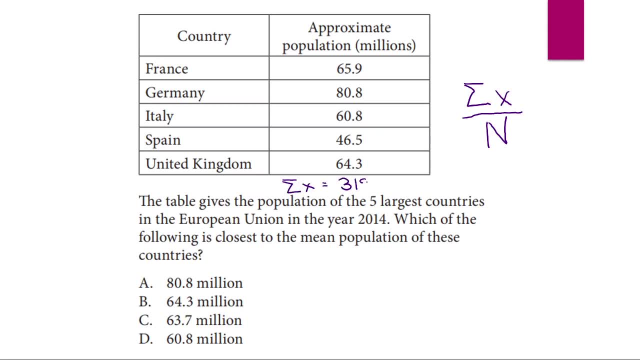 Of all these values Which, if I add all these up, Would give me a 318.3.. Then I'm going to divide that by how many particular countries we have here And notice we have one, two, Three, four, five. 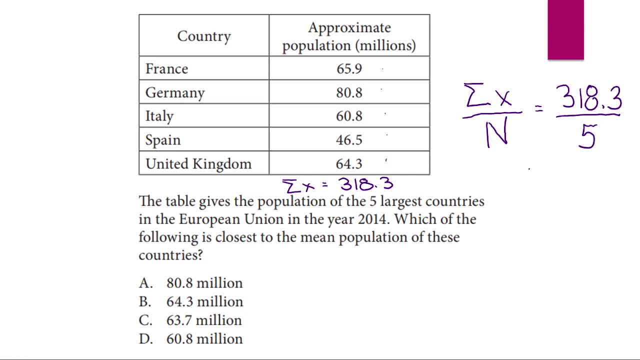 So we're going to divide by five, Which is going to give us a 63.66.. Now, there's not a 63.66 here. We have to round our answer to the tenths place. So remember that means we're going to look at the guy next door. 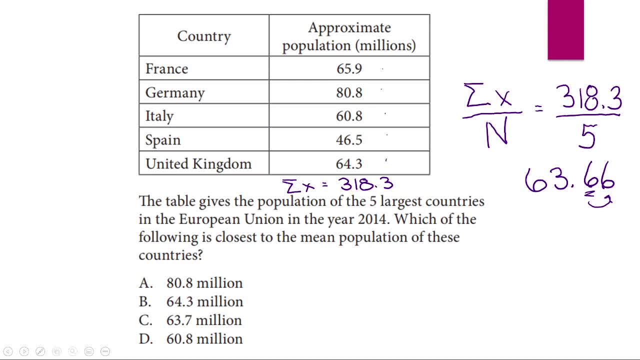 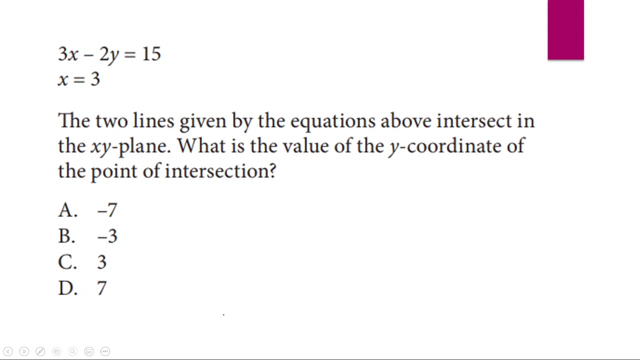 If he's five or more, round up. If not, keep it the same. So our answer in this case becomes 63.7.. Which means for this one, C would be our answer Now. things like this, Okay, Alright. 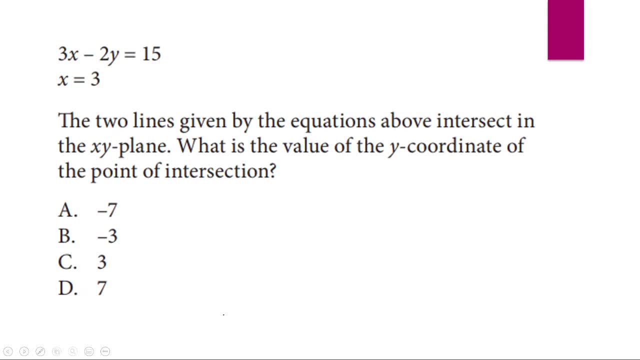 We know that two lines are given by the equations above. We need to know the value of the Y coordinate of the point of intersection. Alright, This means that what we're going to end up doing Is we're going to take this: X equals three. 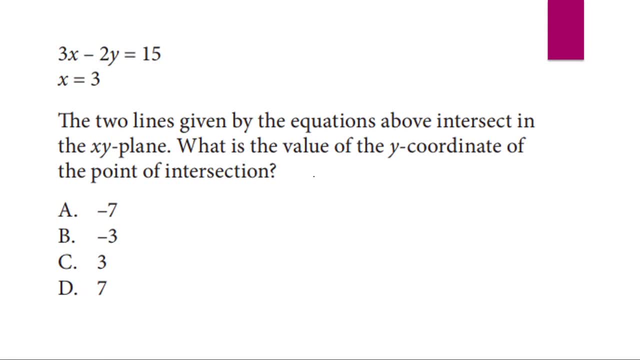 And substitute it into the equation above. So our original equation Is this. Now we're going to substitute in the three, So I have nine minus Two Y, So it should be an equals Equals 15.. Now we need to solve for the Y. 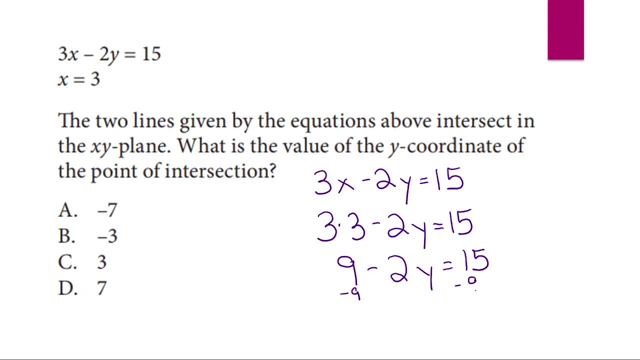 So that means we're going to subtract a nine from both sides, So I have negative two. Y equals 15 minus nine Six. We're still dividing by negatives, Which means my answer here Would be: Y equals Six divided by a negative two. 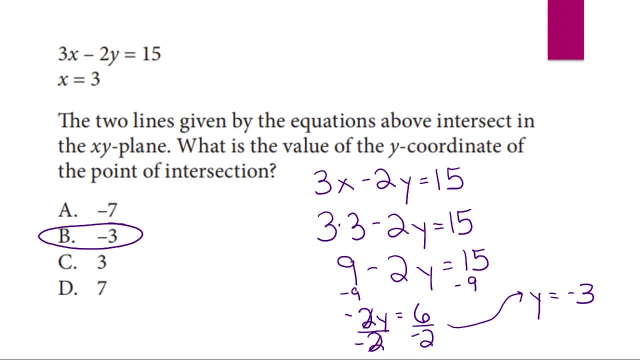 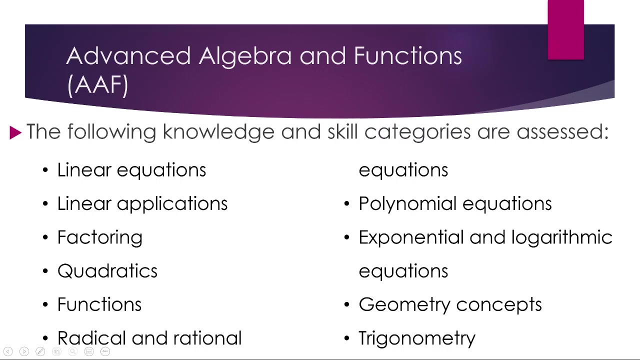 Or negative three. Okay, So you're going to see a lot of problems within this section That are going to be more basic type things Like I said: Algebra, Geometry, Things like that. For the advanced algebra and functions, You're looking at things that you would have seen. 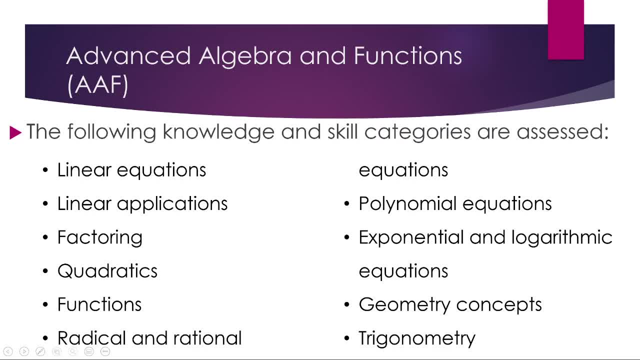 In an algebra two class, A trade class, Things like this. All right, So you're looking at your linear equations, Applications, We're factoring. now We're dealing with quadratics, We're dealing with functions, We're dealing with radicals and rational equations. 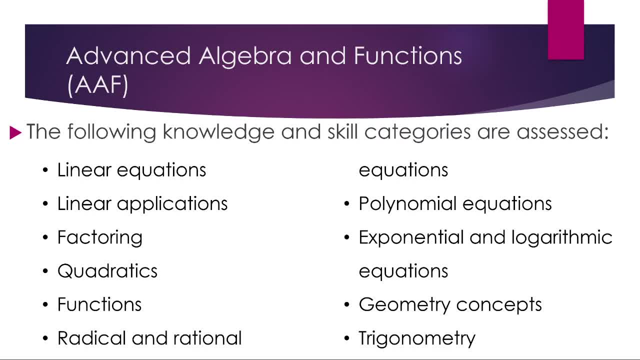 Polynomial equations: Okay, Dealing with your exponential and logarithmic equations, Some general Geometry concepts- Lots of trade can be in here, So you're going to see the things that you would have learned Some of these later math classes. All right, 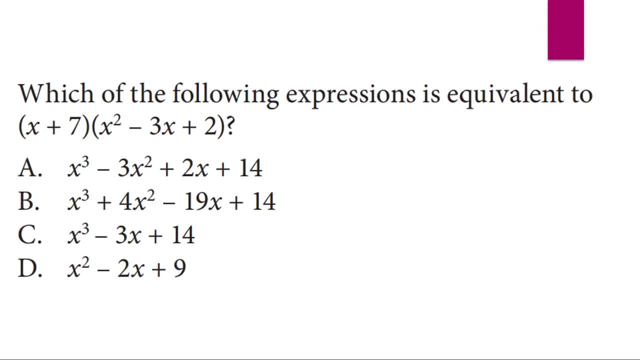 In terms of examples for this. All right, You're going to see things like this, Where we're going to have to find What thing is equivalent to something else. All right, Now one of the things I can tell you, As you do problems like this. 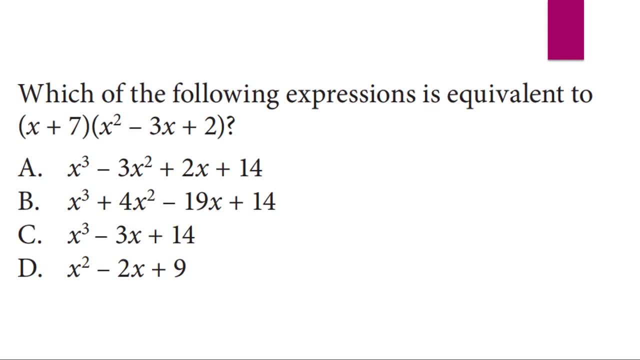 Is you can Work through things And you can start eliminating things That you know right off the bat would not work. So, for example, here I know I'm going to start With- I have to Multiply these two values together. 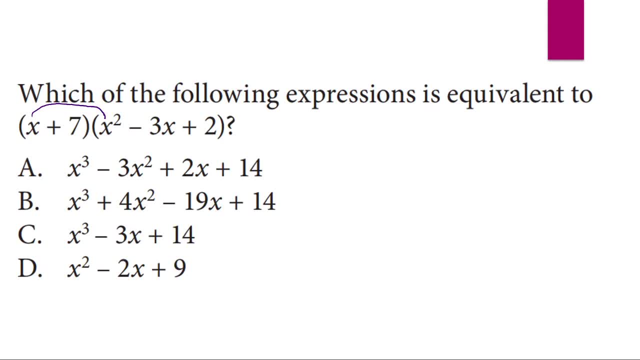 The X And the X squared. Well, when I do that, Then what's going to happen is An X times an X squared Is going to give me an X cubed. So I know that this answer right here That doesn't have an X cubed in it. 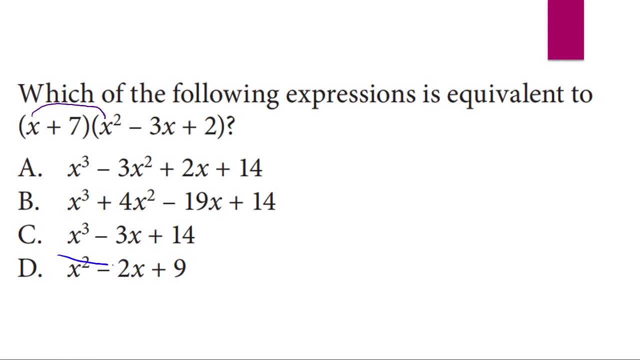 Definitely will never work. So that one's gone All right. I also know That I have to take an X Times a three X, Which is going to give me an X squared. But If you look here At C, 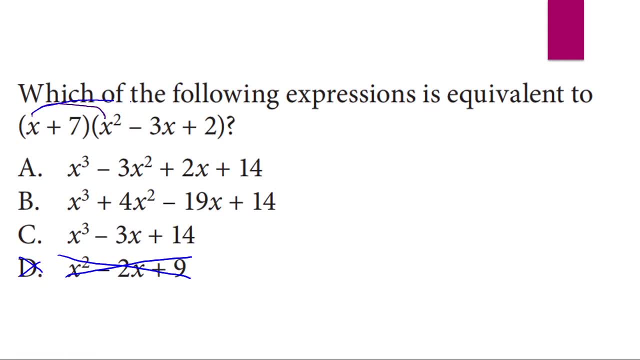 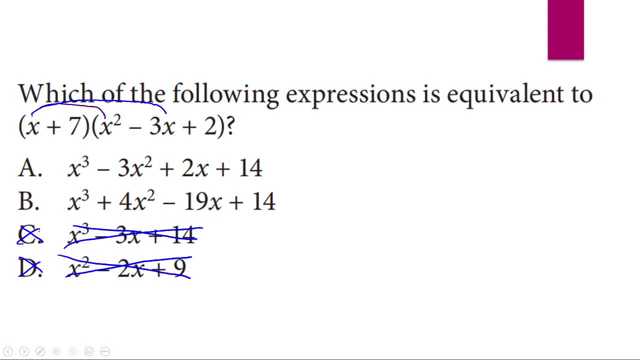 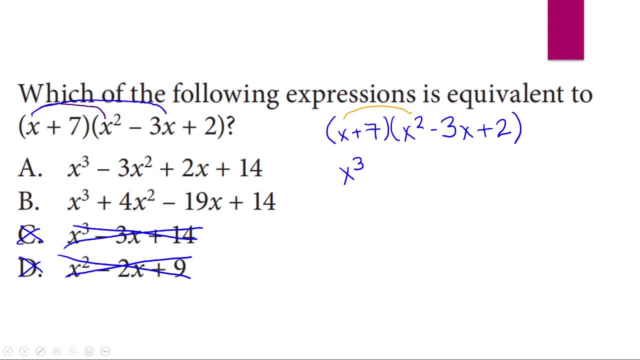 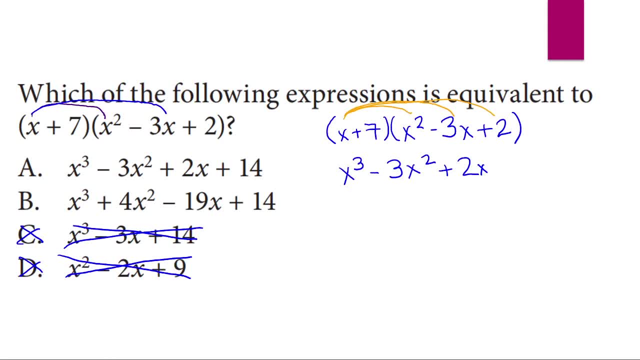 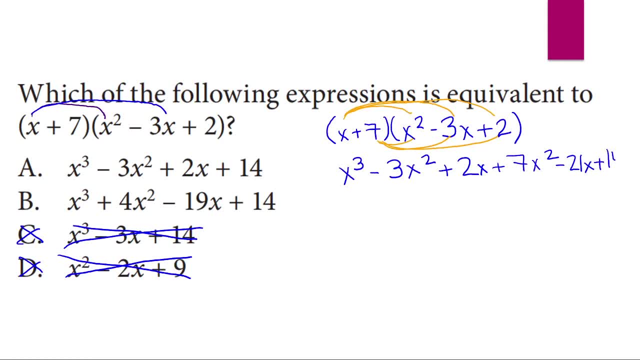 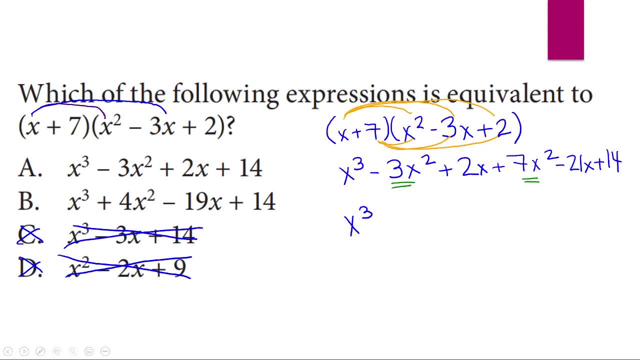 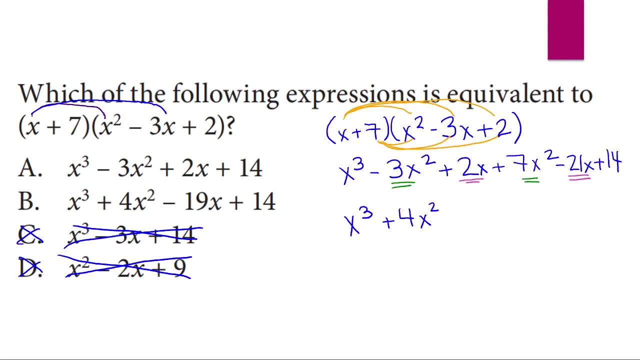 to go together. So it's going to be 2 minus 27,, which gives me 19.. Keep the sign of the larger, So I have a negative 19x And I finish up with a 14.. So if I look O, B would be. 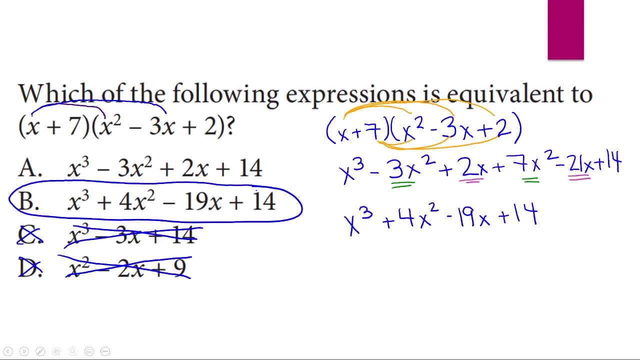 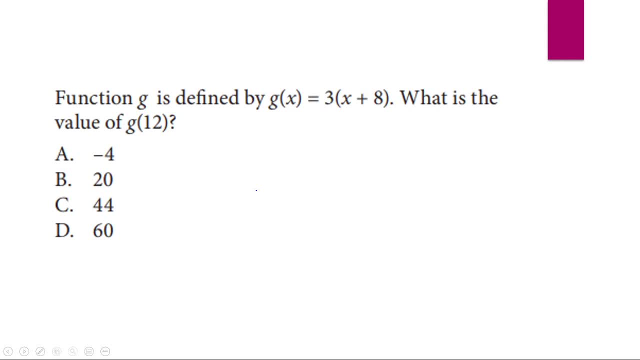 my answer there. This guy is getting into your basic functions. So when you're dealing with your functions- So we know this is what the function says- We want to know what is the value of g of 12.. So if we started off with this guy, when we write things like this, this means that 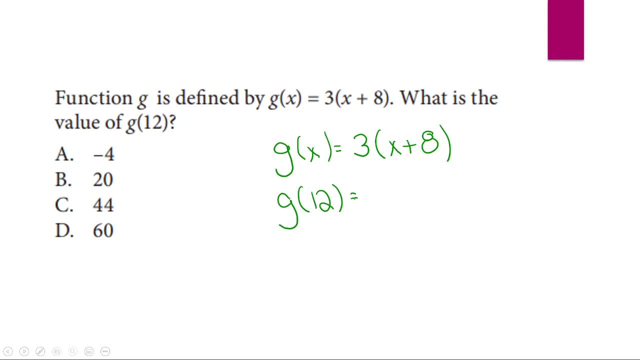 any x that would happen to be in the equation is going to be replaced with a 12.. So I have a 12 plus an 8.. Now remember that everything in math basically boils down to order of operation. All right, so order of operation says I have to do the parentheses. 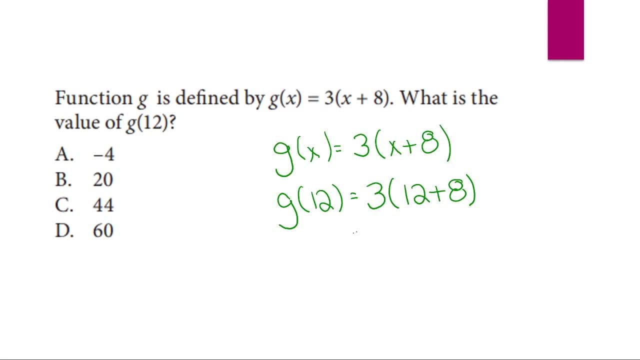 first. So that means I'm going to add these two guys together. So that means I'm going to take 12 plus 8.. What's your answer? 12 plus 8.. Okay, Okay, Which gives me 20.. All right, That 3 is multiplying. So now we're going to go 3 times 20, which? 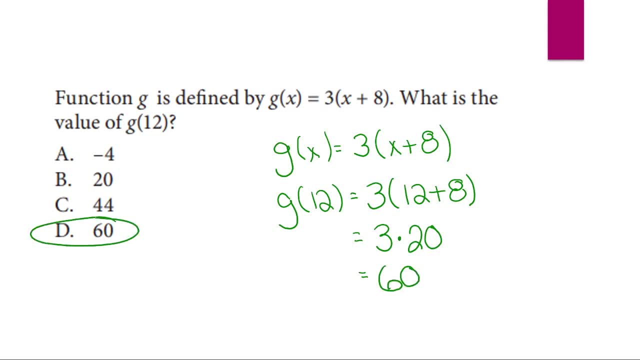 gives me 60. So my answer there is 60.. Now, looking at this, okay, right away, if I would have really wanted to, I would have noticed everything in here I have is positive, which means that finding an answer that's. 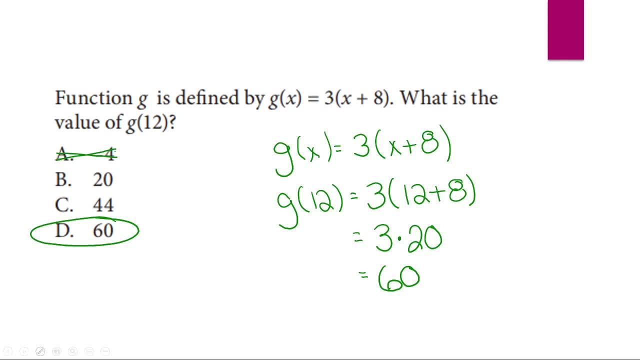 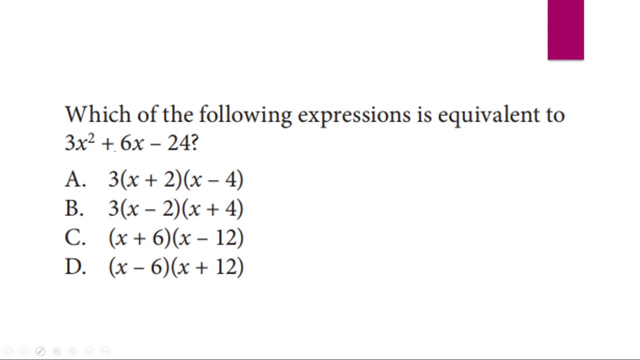 a negative doesn't make any sense to me. Okay, So it's always important to get rid of the things I don't have to consider when I'm taking a test like this. Okay, This guy. I liked this guy in part because I can start really simplifying existence by just looking. 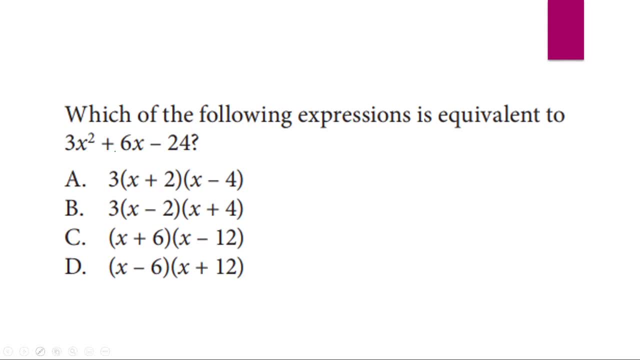 at what am I dealing with here? Okay, So I'm looking for something equivalent to this: 3x squared plus 6x minus 24.. All right, Well, I know, by basic foiling rules, I'm going to end up having to multiply the 6 and this 12 together. Well, I know a negative 6 times. 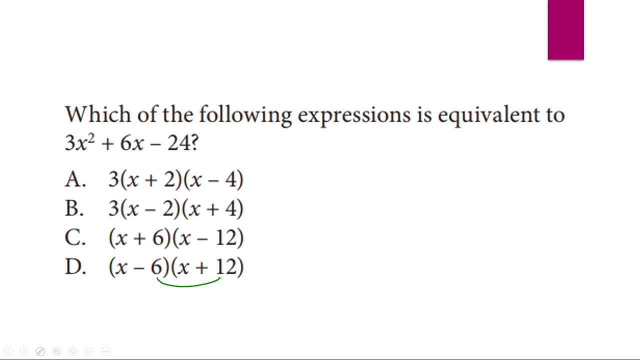 a positive 12 is going to give me a negative 72.. Okay, But I'm looking for a negative 24, which means this guy is definitely out. So is C, because he's going to get a negative 7, because he's also going to end in a negative 74.. Okay, Now we're down to these two guys. 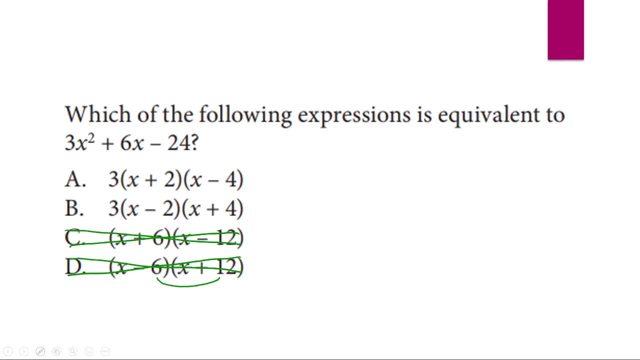 Okay, So let's stop for a second and look at what we can do here with them. So this first one is this: So if I do FOIL, I'm going to get a negative 7. Okay, So I'm going to. 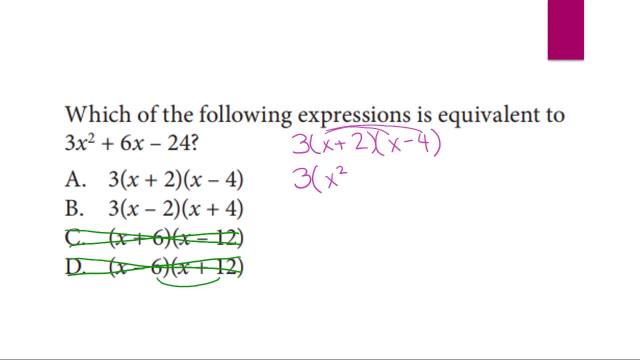 get a negative 7.. Now, let's see if I can figure something out. I can be sure. Okay, What are we going to use? I'm going to use this. So, on behalf of the 2 here, we're looking for a negative 6 squared. Okay, So this would give me an x squared minus a 4x, plus a 2x. 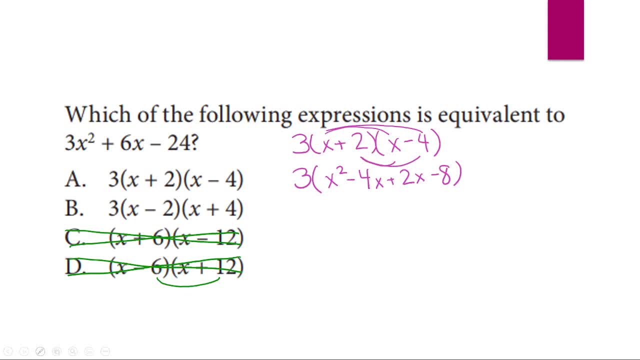 minus an 8.. Well, right off the bat, here I'm seeing a problem, because when I combine these two guys I'm going to get a negative 2 x minus a 4x minus a 2x- fermions that will. 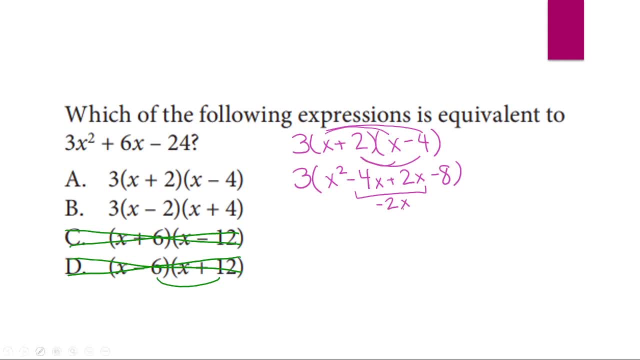 have an equivalent of 8.. Well, now, when I'm doing my 2x, two guys over the second Г. Okay, This is already counter每 1.. said I want a positive, so that means this guy it's also definitely out, it's. 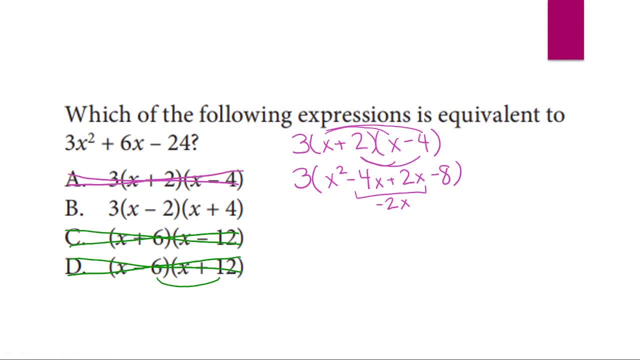 kind of leaves me with one person, and it's always a good thing. just double check to make sure your brain and and your process here equivalent. so I have a negative three times this. so once more, if I do foil, it's an x squared plus a 4x, minus a 2x minus an 8. I can combine these two guys. 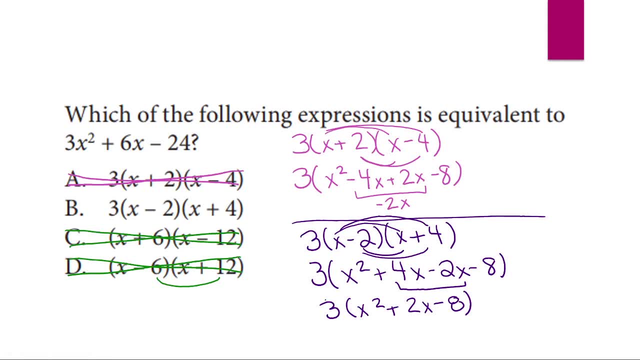 to get a 2x. now we're just distributing this 3, which gives me a 3x squared plus a 6x minus 24, which is what I actually want. okay, so that just kind of helps verify that I do have the correct answer here. all right, one more here, all right. 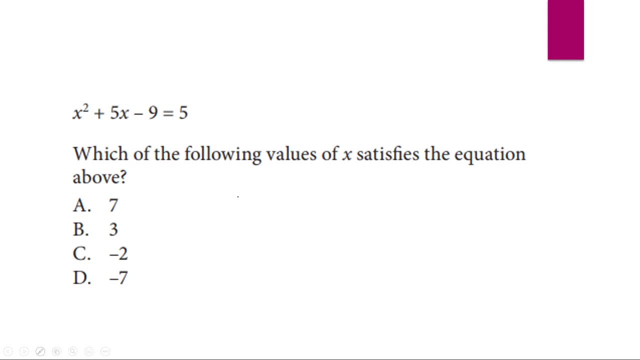 this guy. okay, I need to know which of the following value satisfies the equation, okay, well, if you're looking at this here, there's a few things right off the bat we can get rid of, alright. for example, if we started with a positive 7, well, that's. 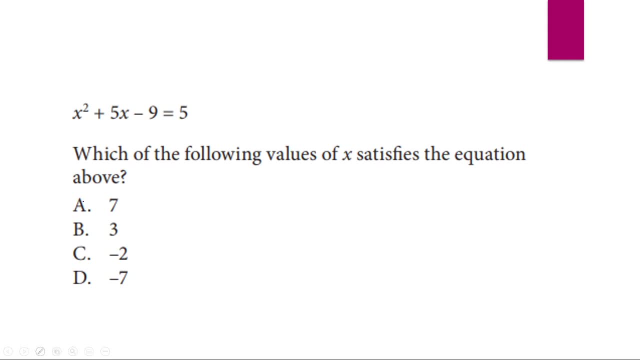 going to give me a 49 plus a 35, which is definitely larger than 5, so I know that guy isn't going to work. for the next one, I'm going to get a 9. the area I'm subtracting a 9, which means I'm only going to be left. 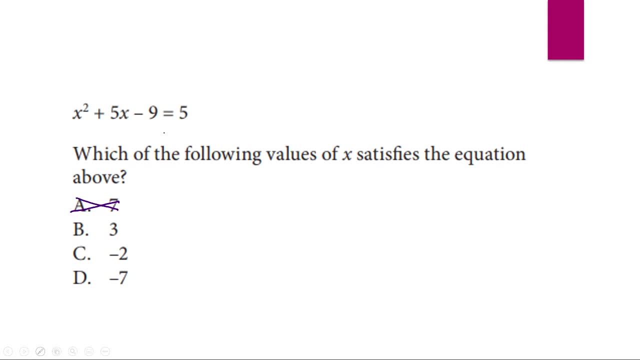 with that 5 times 3, meaning 15, that's not going to work. if I do the negative 2, hmm, that could possibly work. but notice something: if I do a negative 2, I would be ending up with negative 2 squared, which is 4,. 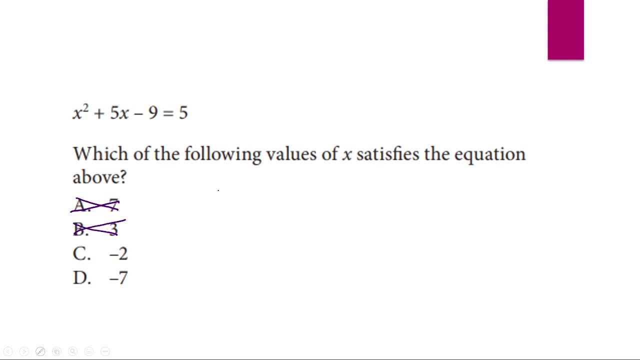 and negative 4 theta and negative 3 over there because that's going to kill every random number. But then I go 5 times: a negative 2 gives me a negative 10 and I had a negative 9.. Oh, massive negative answer there. That's not going to work. 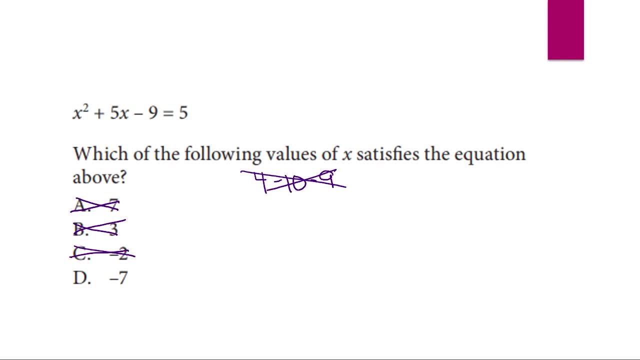 Alright, so let's see if the guy I think's going to work is going to work. So we have a negative 7, it's squared plus. we have 5 times a negative 7 minus a 9.. Well, I know a negative number squared is going to be a positive number, so it's going to be a positive 49.. 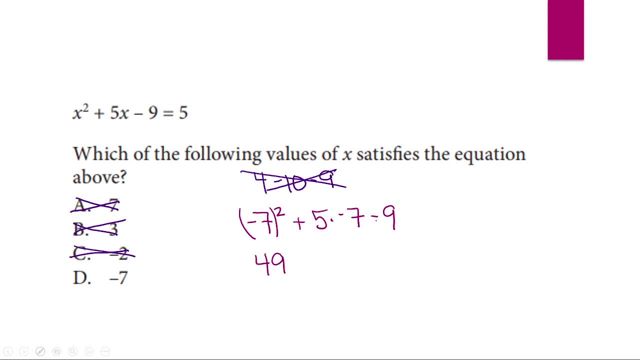 A 5 times a negative 7 is going to leave me with a negative 35 minus 7.. That's 9.. Okay, well, a 45 minus a 35 minus a 9 leaves me with 5, which is what I wanted here. 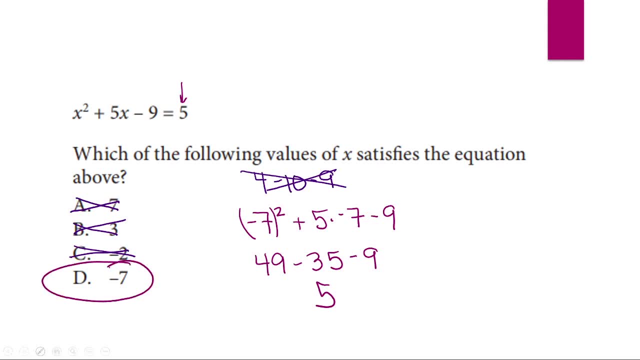 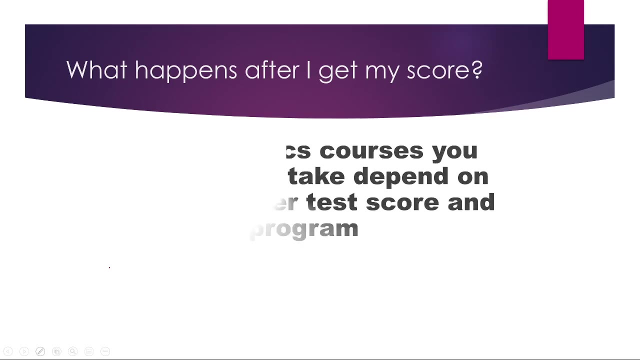 So this would be my answer here. Alright, sometimes the process of elimination and just thinking kind of mathily will help us along here. Alright, If you want to score, please note okay where you go in. math depends not only on your test score but also on your degree program. 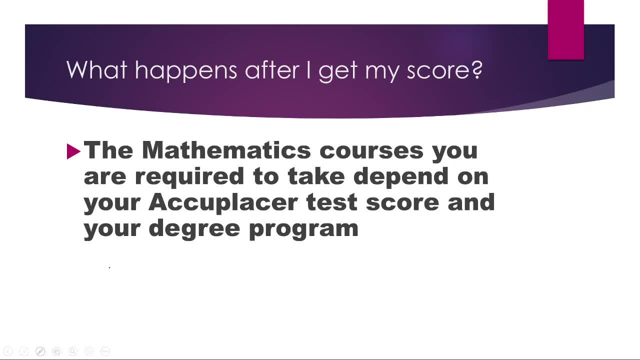 Alright. The key, though, is you want to score as high as possible, because you do want to be able to finish up your math without doing a bunch of extra remedial math courses. So don't just go in and go, ah, math, whatever, okay, and blow it off. 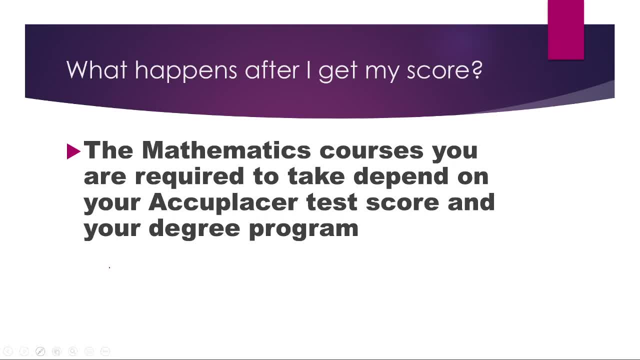 You want to score the best you can, Alright. One thing that I encourage people to do is, once you take the mat, the Accuplacer math portion, you see what your test score is. you know what your degree program is. talk to your advisor about what courses do you need to take? 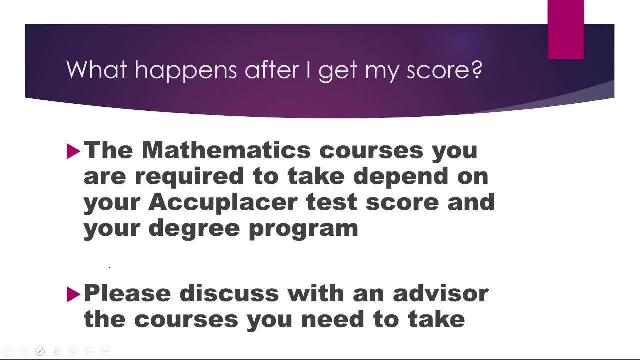 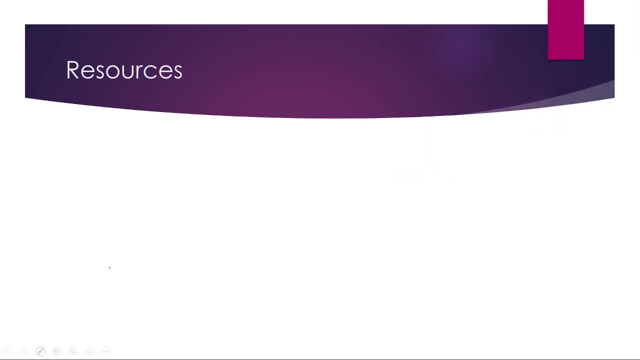 Alright, That way you get started on the correct road. Please don't take the math and just kind of blow it off and I'll do it later, because that does end up with problems in the future. Okay, If you're looking for, how exactly am I going to prepare for this? here's some basic resources.